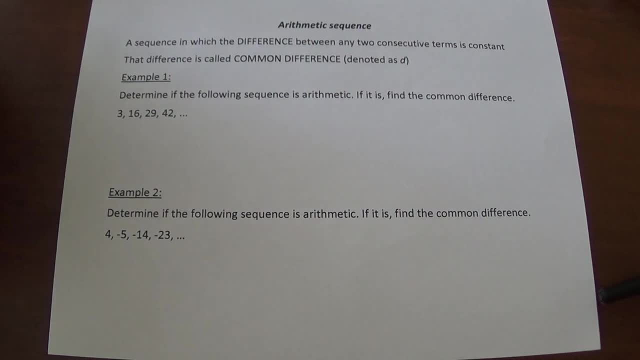 Hi, today we are going to talk about something called arithmetic sequence. So we define arithmetic sequences as sequences in which the difference between any two consecutive terms is going to remain constant And that difference is going to be called common difference and we denote it as D. So we're going to take a look at several examples where we need to 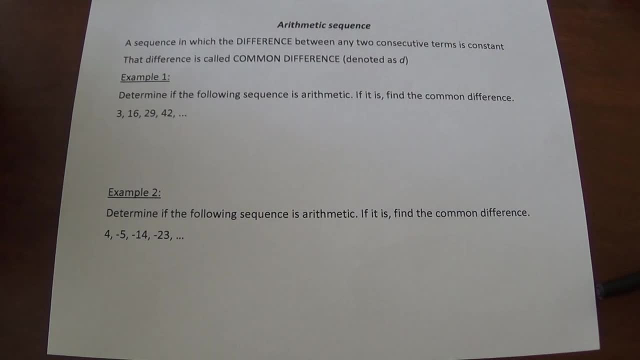 determine if a sequence is an arithmetic sequence. If we take a look at example 1, it's asking us to determine if the following sequence is arithmetic and if it is to find the common difference. The sequence is 3,, 16,, 29,, 42, and so on. So what we need to do is we need 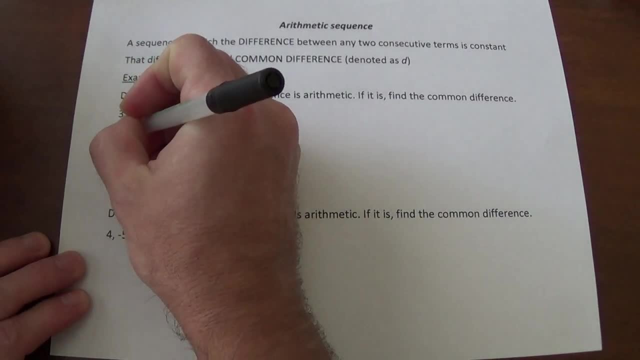 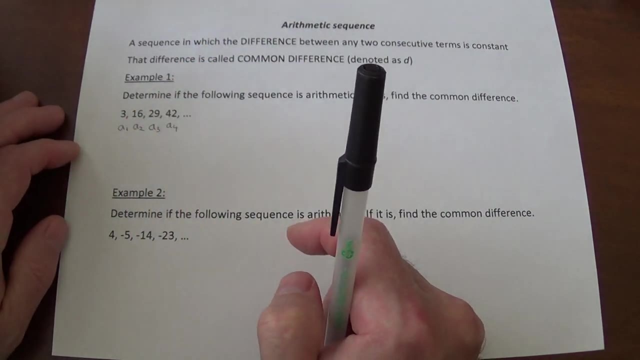 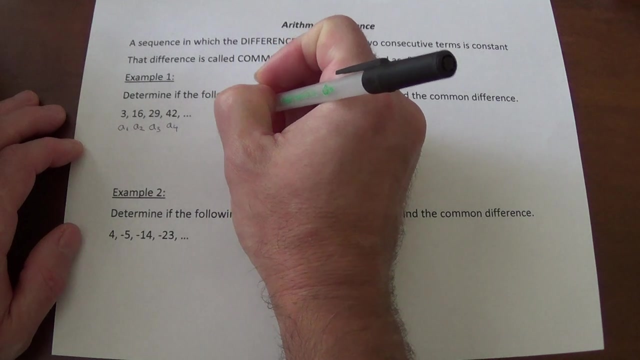 to understand, first of all, that this is going to be our first term, this is our second term, this is our third term, this is our fourth, And what we need to do is determine if the difference between consecutive terms is going to stay the same. So we're going to take the difference between the second term and the 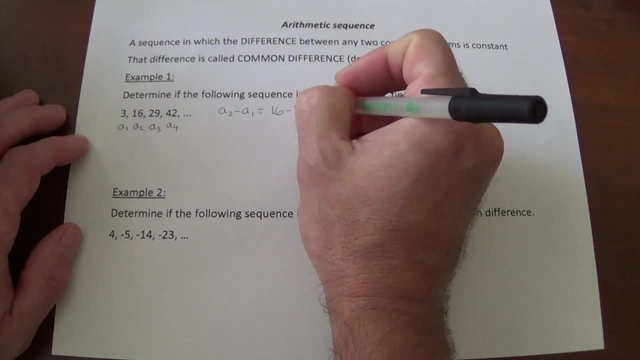 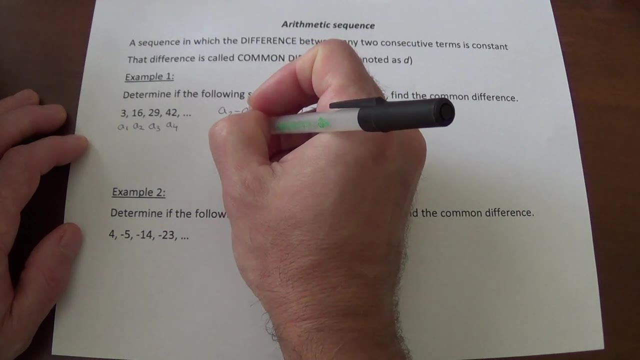 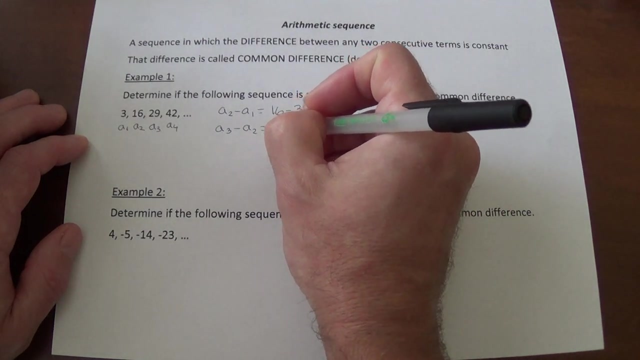 first term, which in our case is 16 minus 3, and that is 13.. Then we're going to take a look at the difference between a3 and a2, which is the difference between the third term and the second term, and that's 29 minus 16.. 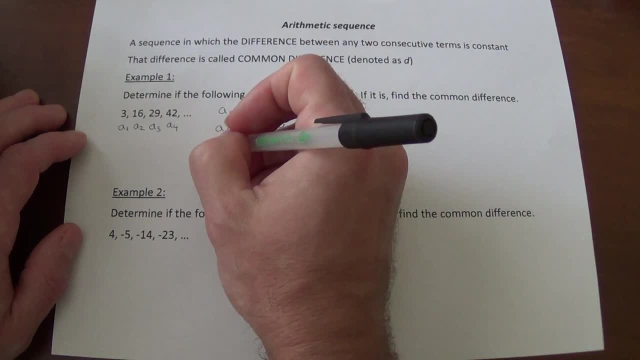 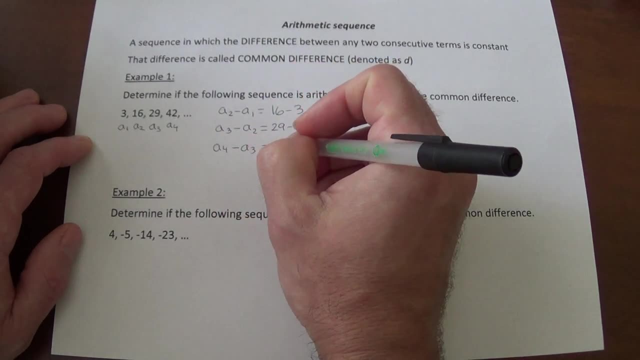 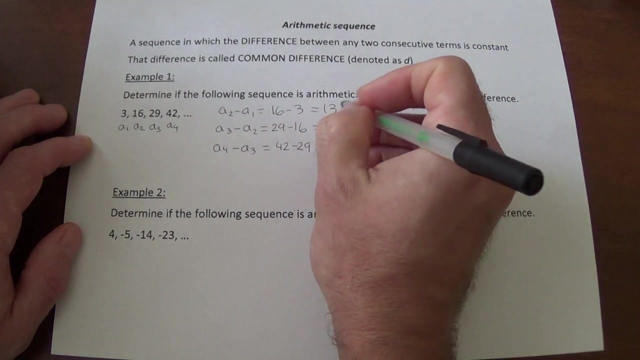 And that is 22.. And that is 13 also. And finally, we're going to take the fourth term minus the third term, which is 42 minus 29,, and that is also 13.. So, for all these differences, we got 13.. 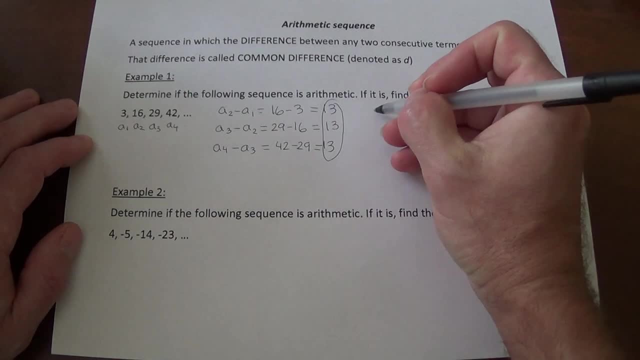 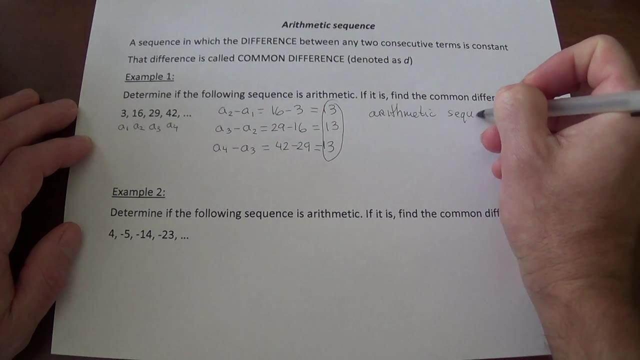 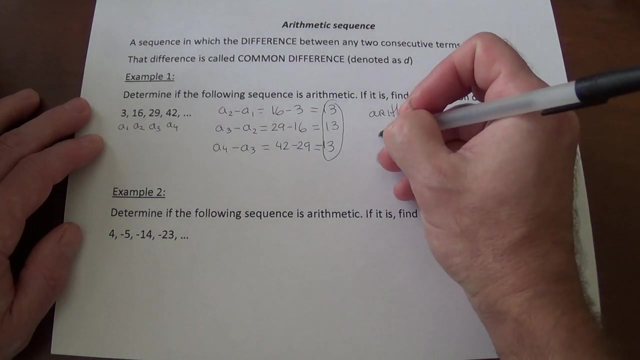 Since the difference remains the same, we can conclude that this is an arithmetic sequence, And then the common difference is actually going to be that number that we found here. So the common difference in this case is going to be 13.. And we're done. 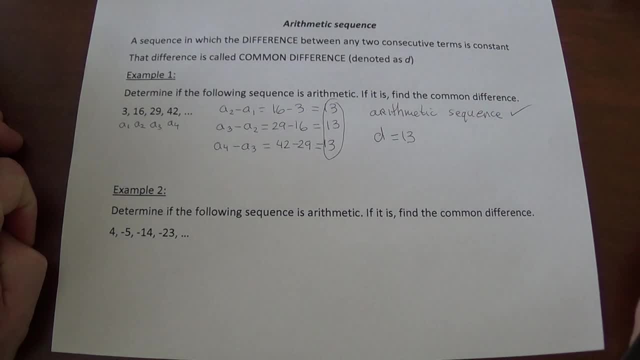 So what we're going to do now is take a look at the next problem, Same exact question, except our sequence, obviously, is going to be different. So our terms are 4, negative, 5, negative, 14, negative 23.. Okay, 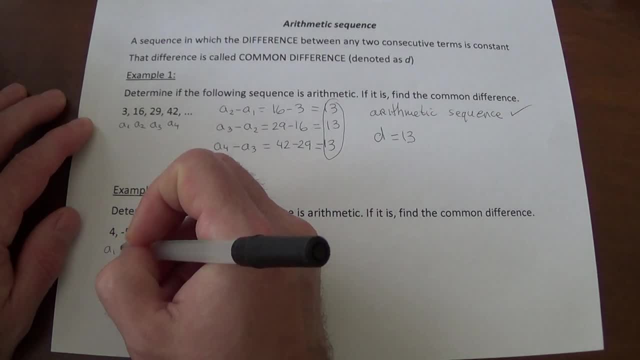 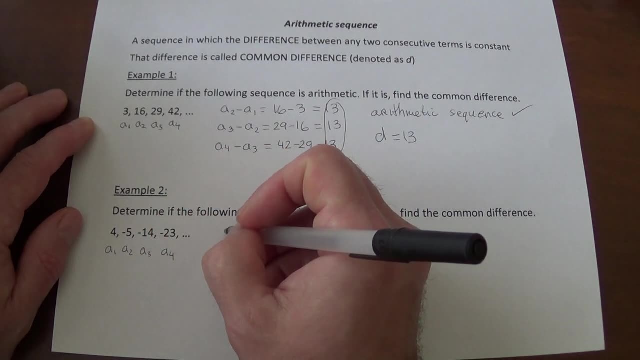 And we are going to follow the same process. We're going to understand that this is the first term, this is the second term, this is the third term, this is the fourth term. So, following the same process, a2 minus a1 is going to be negative, 5 minus 4, which is: 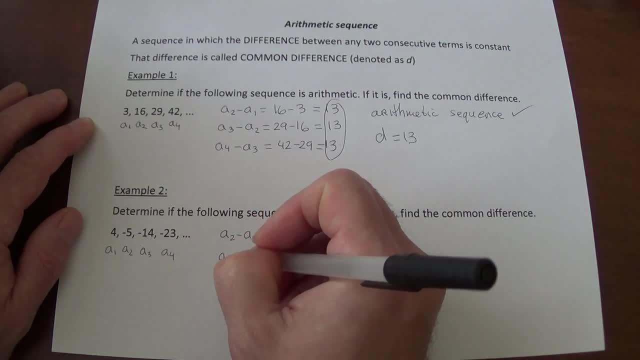 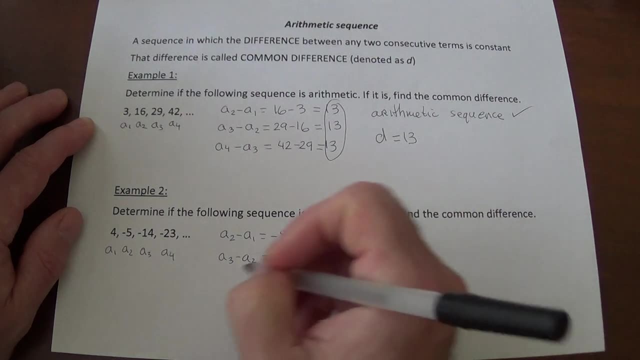 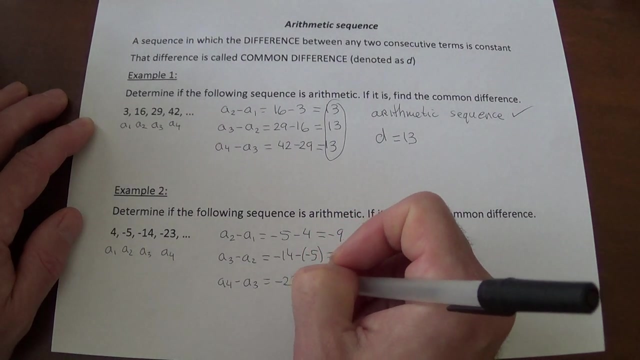 negative 9.. a3 minus a2 is going to be negative 14 minus negative 5,, which is also negative 9.. Okay, Okay, So a2 minus the third term is going to be negative 23 minus negative 14,, which is also. 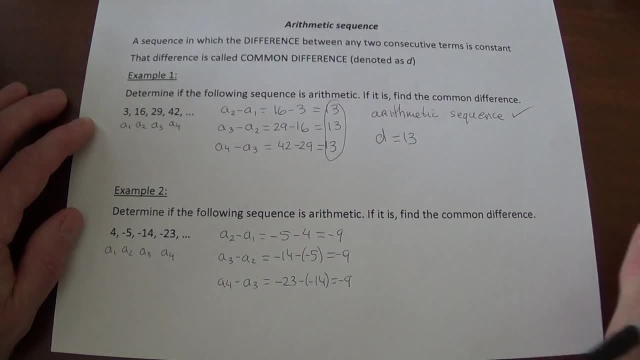 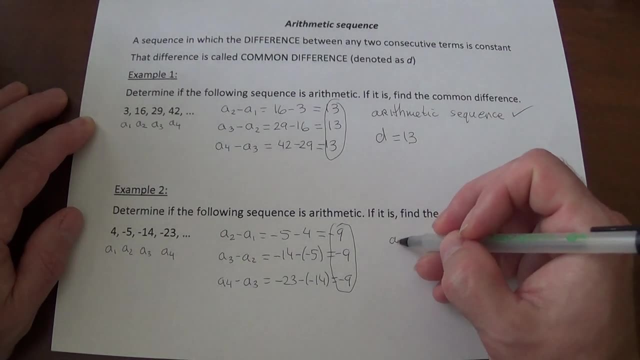 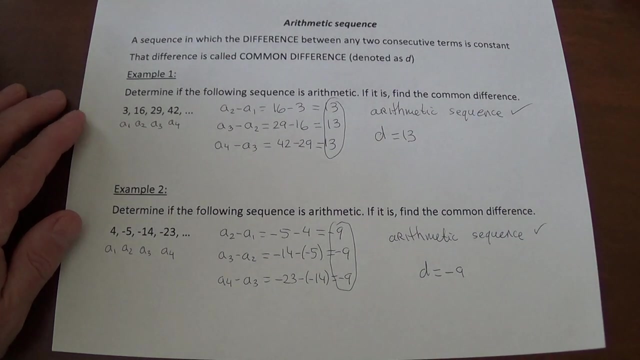 negative 9.. We have the same difference- negative 9, when we subtract consecutive terms And then we conclude that this is an arithmetic sequence, And then the common difference will be, as you probably already guessed, negative 9.. I have a couple more examples for us to look at. 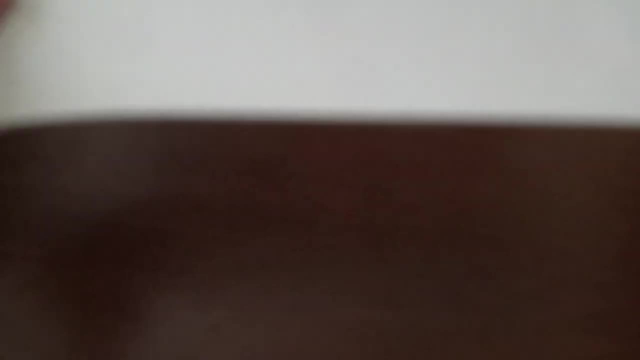 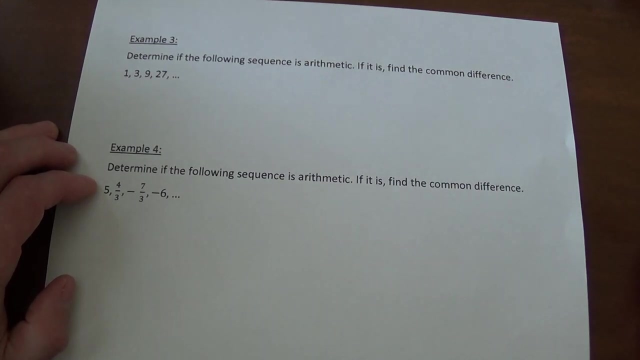 Same exact question. So example 3.. Determine if the following sequence is arithmetic. If it is, find the common difference. The sequence is 1, 3, 9, 27.. Some of you may probably recognize some kind of a pattern here, which is good. 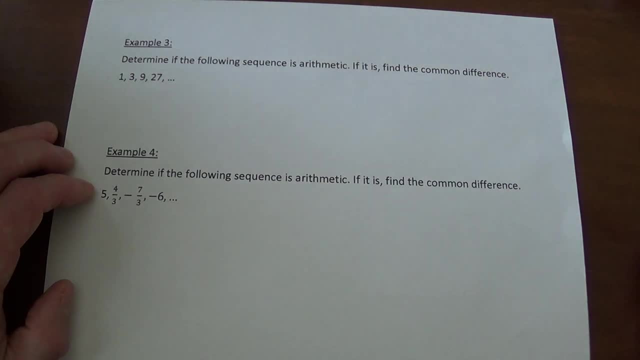 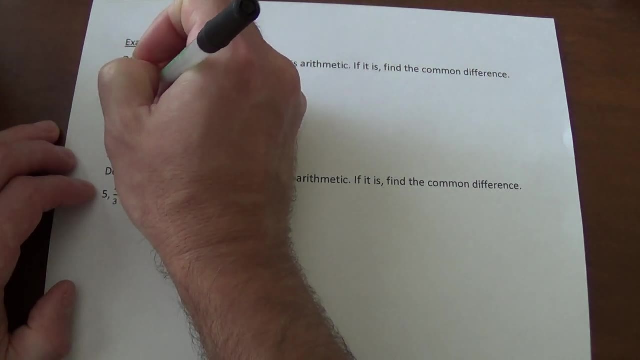 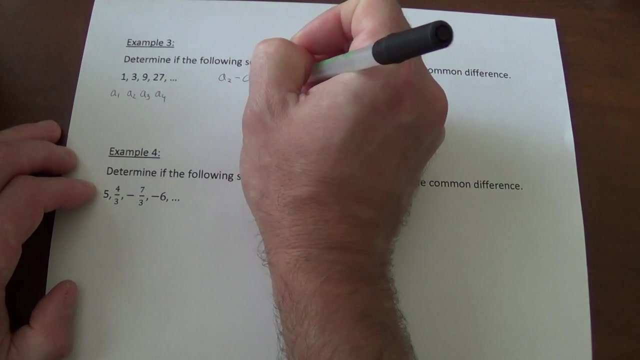 Although we are interested in determining the specific pattern. So if we identify this as the first term and the second term, and the third term and the fourth term, and we find the difference between the second term and the first term, that's 3 minus 1.. 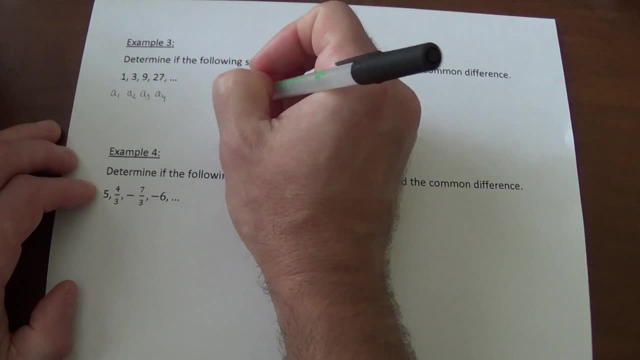 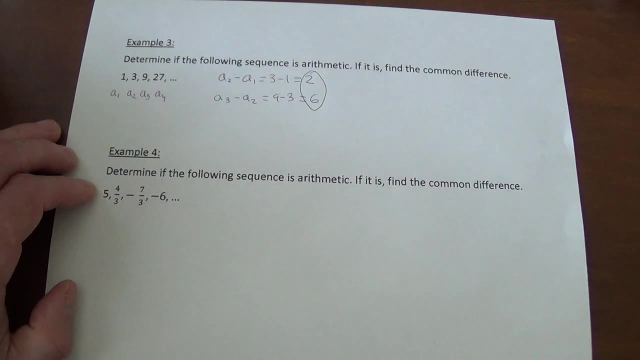 That's going to give us 2.. The third term minus the second term is 9 minus 3, is going to give us 6. And, unfortunately, Or 4. Or fortunately, but we already have a problem Because these terms, these two differences, don't match. 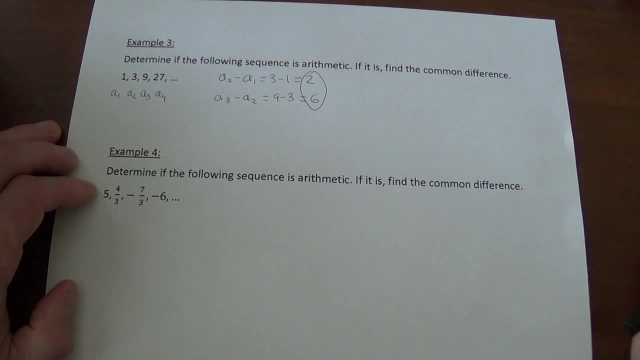 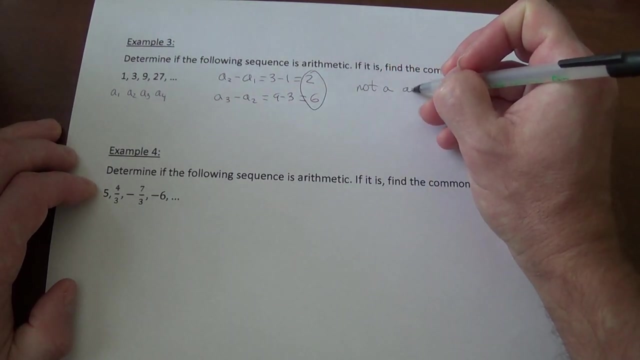 And if they do not match, then it doesn't really matter what happens. if I try to do two more terms, That means that our difference is not going to stay the same and this is not a common difference. I'm sorry, not an arithmetic sequence.